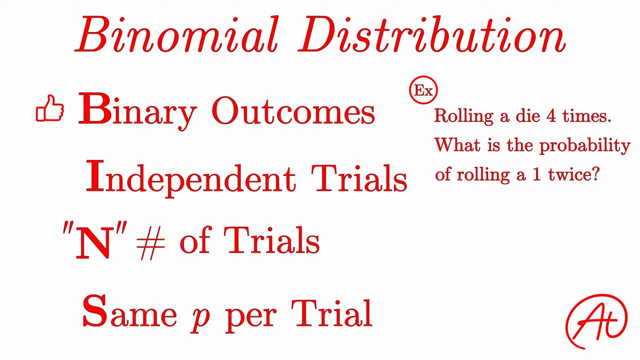 number during one trial has no effect on the number you roll on the next trial, so this also satisfies the I. Then we are rolling the die four times, so we specifically have four trials and that satisfies the N. And finally, during each trial we have the same probability of one sixth for rolling. 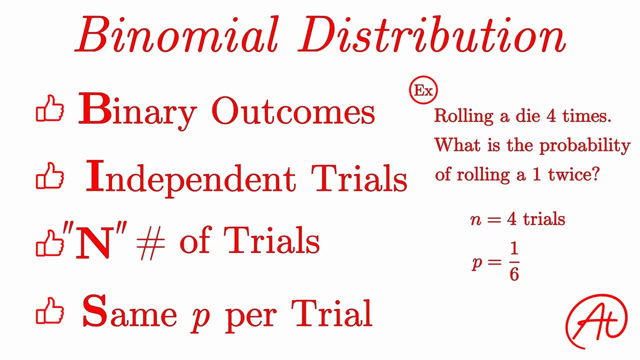 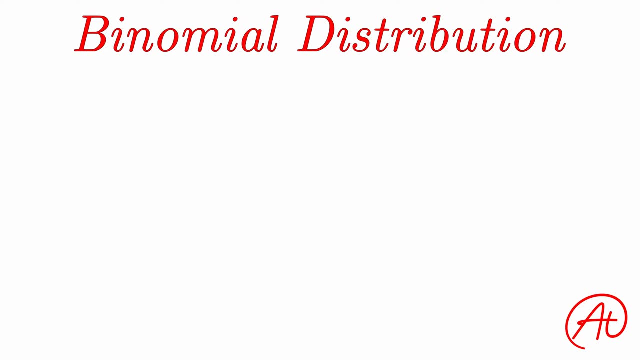 a 1, so that satisfies the S. And because all these conditions were met, we know this experiment will follow a binomial distribution. Now that we covered what makes something a binomial distribution, let's go over some properties of this distribution. First, the mean or expected value For the binomial distribution. 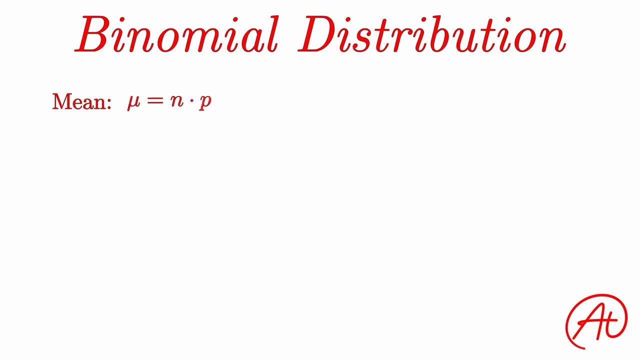 distribution. the mean mu is pretty simple and equals n times p, where n is the number of trials for the experiment and p is the probability of success for each trial. Next, the standard deviation is also pretty straightforward. Sigma equals the square root of n times p times 1 minus p, or you might also see it. 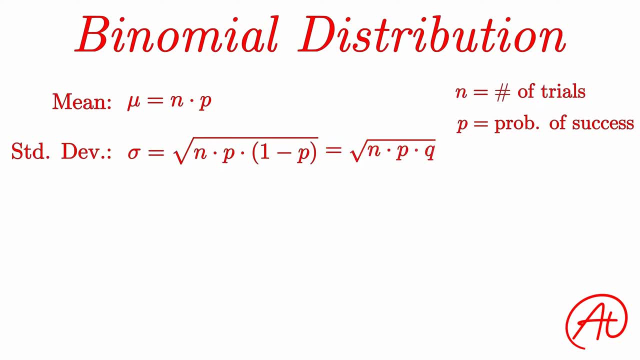 as the square root of n times p times q, where q equals 1 minus p, aka the probability of failure, since there are only two outcomes for a trial. Finally, let's go over some of the more interesting stuff: probability. 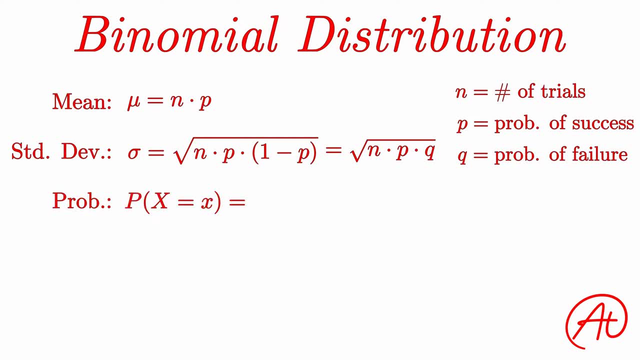 If you want to calculate the probability of getting x number of successes in your experiment, all you do is n. choose x times p, raised to x times q raised to n minus x. Uhhhh, what To see what the heck this means and where it comes from. let's dissect it a bit with. 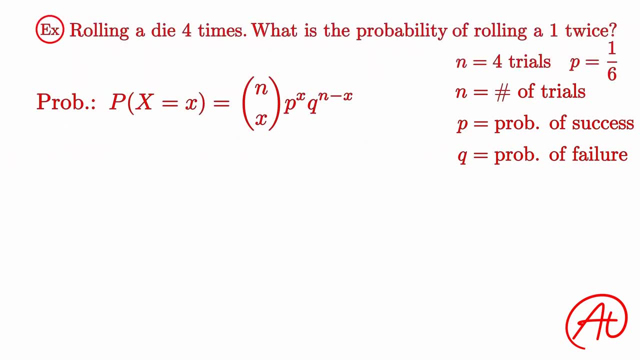 our previous example of rolling a die four times As a reminder. in this experiment we want to find the probability of rolling a 1, two out of our four trials. So first let's look at what this right side of the formula gives us. 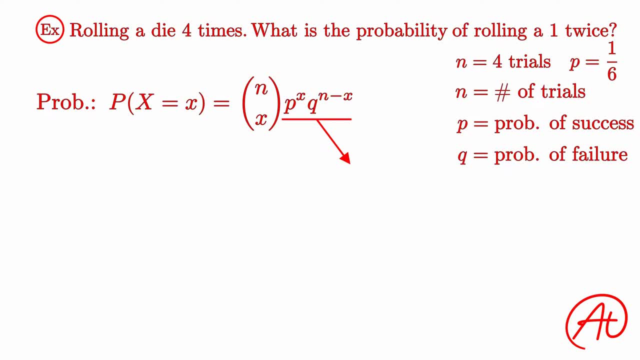 With our n equaling four trials, our probability of success equaling 1 sixth and our die desired number of successes equaling 2,, we can write this as: 1 sixth squared times, 5 sixths raised to 4 minus 2, or 5 sixths squared. 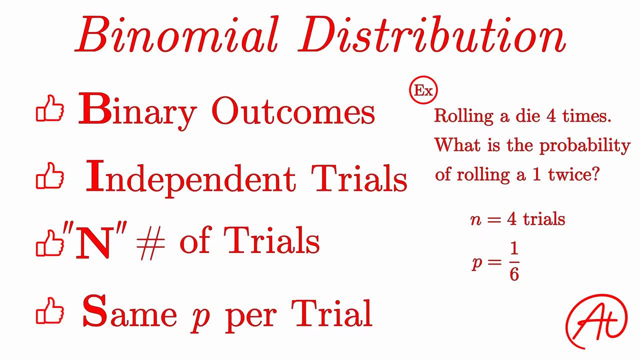 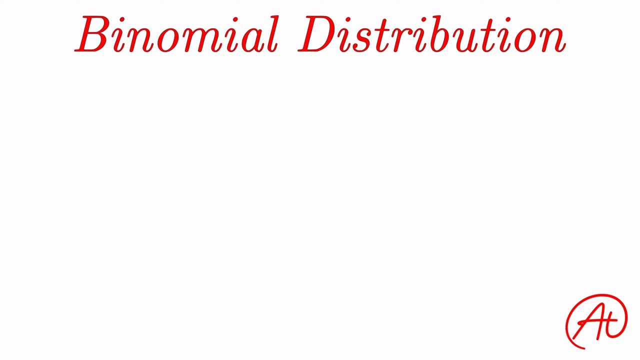 so that satisfies the S, And because all these conditions were met, we know this experiment will follow a binomial distribution. Now that we've covered what makes something a binomial distribution, let's go over some properties of this distribution. First, the mean or expected value For the binomial distribution. 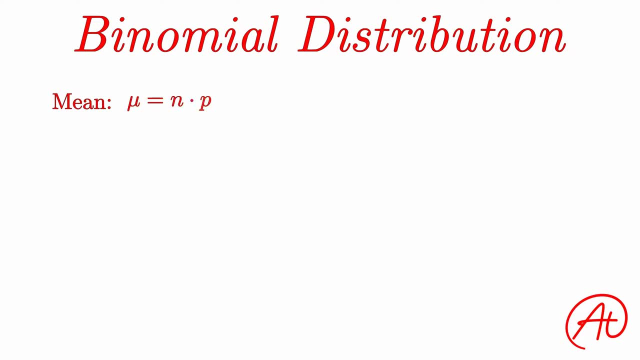 distribution. the mean mu is pretty simple and equals n times p, where n is the number of trials for the experiment and p is the probability of success for each trial. Next, the standard deviation is also pretty straightforward. Sigma equals the square root of n times p times 1 minus p, or you might also see it. 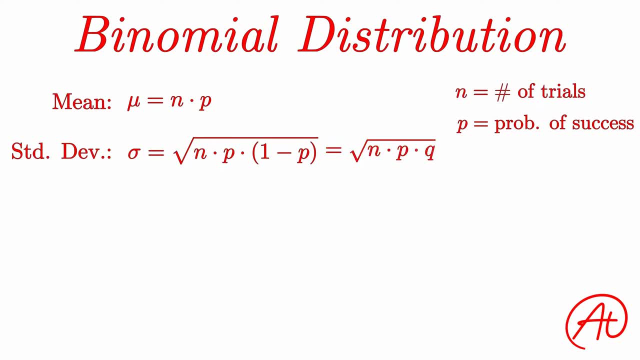 as the square root of n times p times q, where q equals 1 minus p, aka the probability of failure, since there are only two outcomes for a trial. Finally, let's go over some of the more interesting stuff: probability, If you. 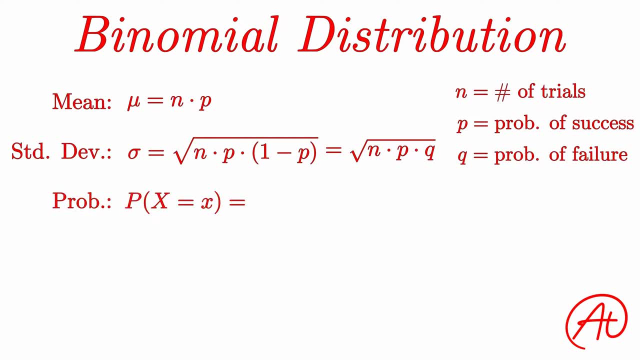 want to calculate the probability of getting x number of successes in your experiment. all you do is n, choose x times p, raised to x times q raised to n minus x. Uh, what To see what the heck this means and where it comes from. let's dissect it. 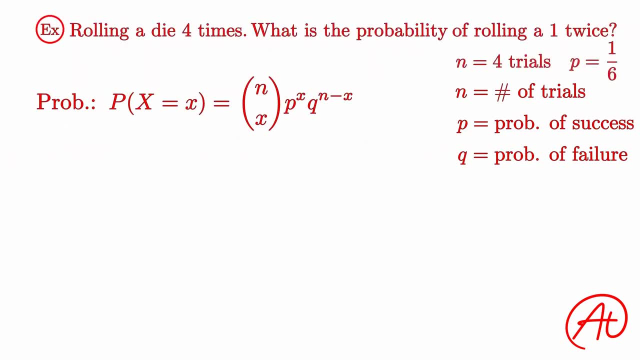 a bit with our previous example of rolling a die four times. As a reminder, in this experiment we want to find the probability of rolling a 1, 2 out of our four trials. So first let's look at what this right side of the formula gives us. 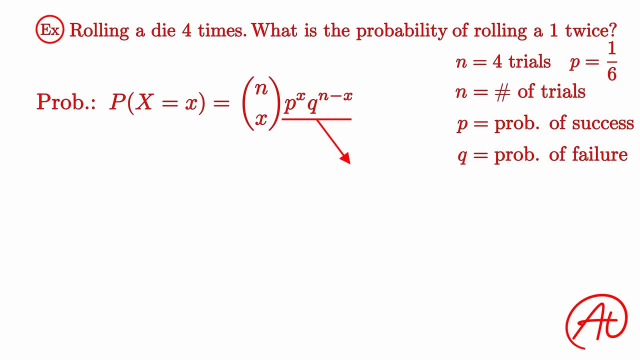 With our n equaling four trials, our probability of success equaling 1 sixth and our desired number of successes equaling 2,, we can write this as 1 sixth squared times, 5 sixths raised to 4 minus 2, or 5 sixths squared If we were to expand. 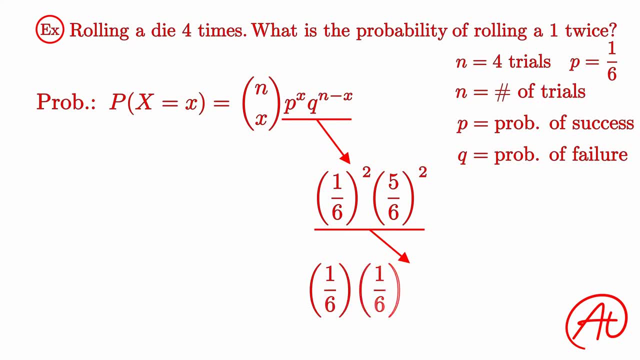 this out. it would be 1 sixth times 1 sixth times 5 sixths times 5 sixths. But what does this mean? Well, since each of our four trials are independent, to find the probability of a certain situation occurring, we can multiply together the probabilities of the outcomes. 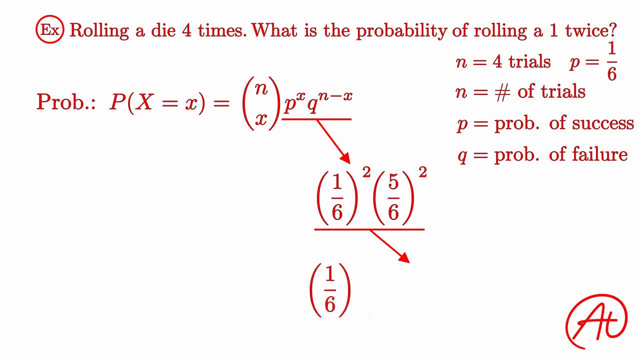 If we were to expand this out, it would be 1 sixth times 1, sixth times 5 sixths times 5 sixths. But what does this mean? Well, since each of our four trials are independent, to find the probability of a certain success, 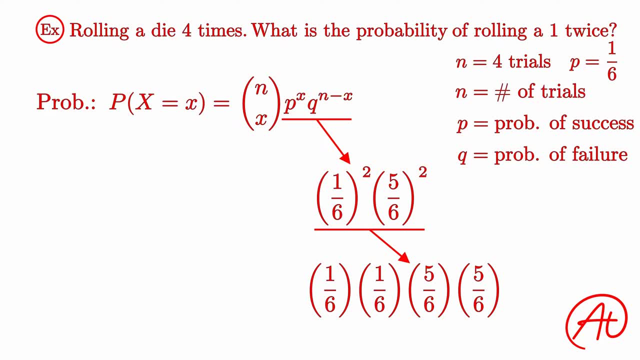 a certain situation occurring. we can multiply together the probabilities of the outcomes for each trial. So, in this order, we would specifically be finding the probability of getting a success: a success on the second roll, a failure on the third roll and then, finally, a failure on the fourth roll. 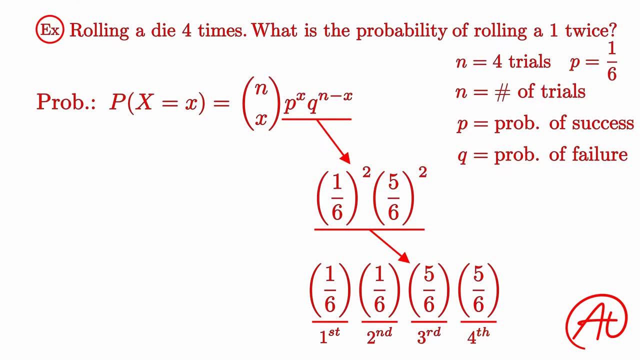 So, essentially, this right side is a way to calculate the probability of one specific situation that satisfies our desired outcome, But there are other situations that satisfy this as well. right, What if we rolled a 1 on our first and third rolls, Or on our third and fourth rolls? 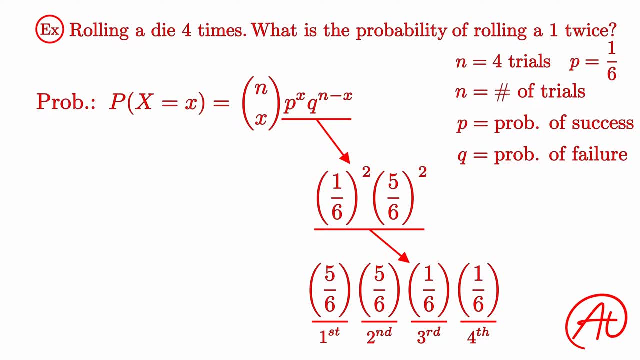 Or any of the other situations that result in two 1s. How do we account for all those possibilities? Well, that's where this thing comes into play, which is pronounced as n choose x. Basically, what this fact says is that if we roll a 1 on our first and third rolls, 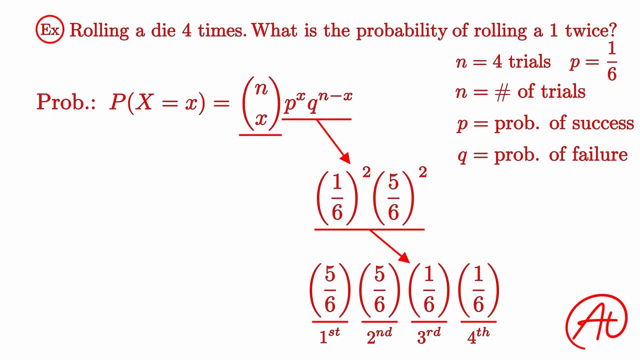 we get a success. What this value gives us is the total number of different ways you can write your desired outcome. In other words, out of our n trials, how many ways are there to have x successes? Or, for our example, out of 4 rolls, how many ways are there to roll a 1 twice? 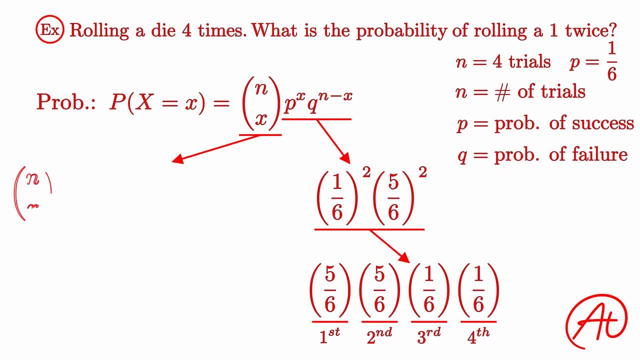 So to calculate n, choose x, you need to look at one more ugly-looking formula. But just like the other one, it's not as scary as it looks. So to calculate n, choose x, you need to look at one more ugly-looking formula. 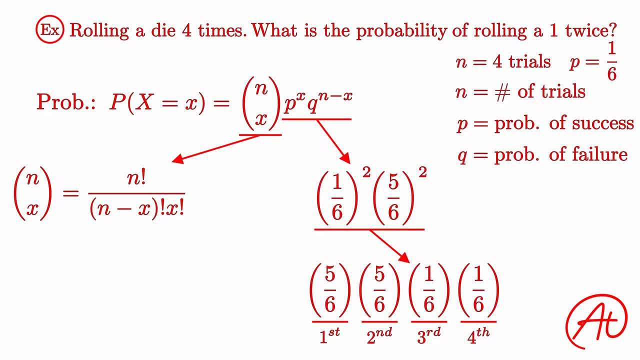 But just like the other one, it's not as scary as it looks. So to calculate n, choose x. you need to look at one more ugly-looking formula, If you haven't seen them before. these exclamation points represent factorials, And all a factorial is is taking a number and multiplying it by each integer below it. 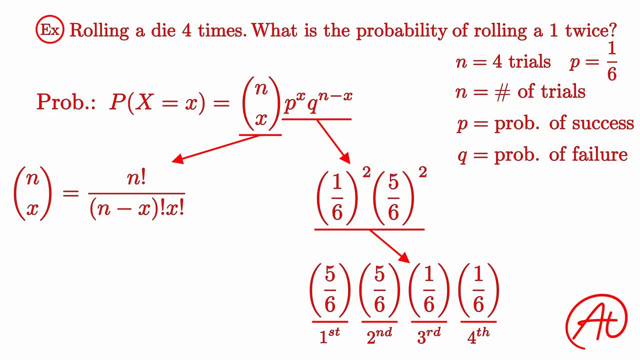 until you reach 1.. So the factorial of 3 would be 3 times 2 times 1, or equal to 6.. And if we wanted to calculate 4, choose 2,. for our example, we would take 4 factorial. 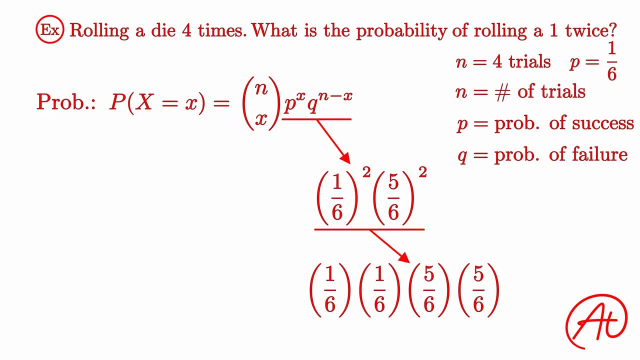 for each trial. So, in this order, we would specifically be finding the probability of getting a success, aka rolling a 1 on the first roll, a success on the second roll, a failure on the third roll and then finally a failure on the fourth roll. So essentially, 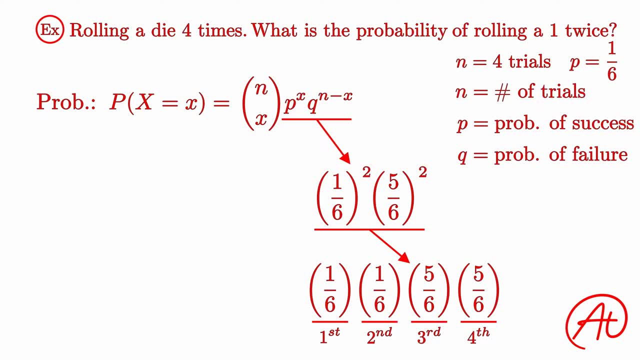 this right side is a way to calculate the probability of one specific situation that satisfies our desired outcome of rolling a 1 twice. But there are other situations that satisfy this as well. right, What if we rolled a 1 on our first and third rolls, Or on our third and fourth rolls, Or any of the other situations? 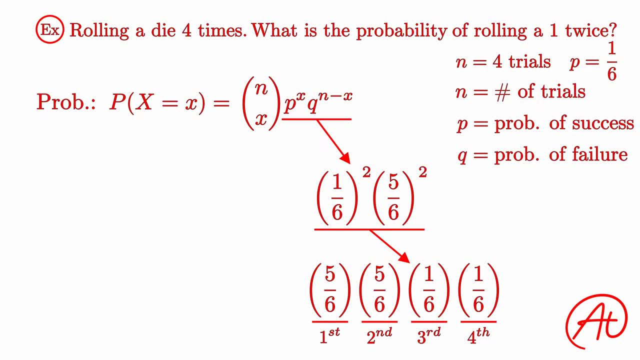 that result in two 1s. How do we account for all those possibilities? Well, that's where this thing comes into play, which is pronounced as: n choose x. Basically, what this value gives us is the total number of different ways you can write your desired. 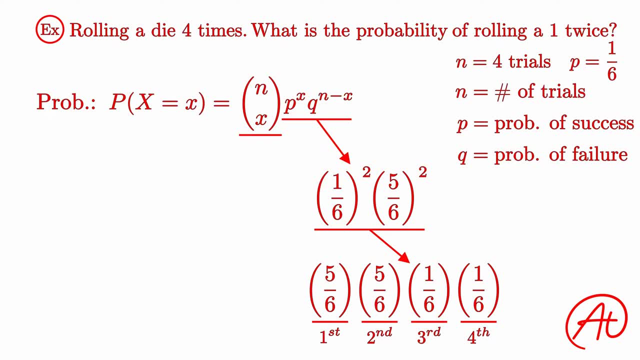 outcome. In other words, out of our n trials, how many ways are there to have x successes? Or, for our example, out of 4 rolls, how many ways are there to roll a 1 twice? So to calculate n, choose x. you need to look at one more ugly-looking formula, But just like the other one, it's. 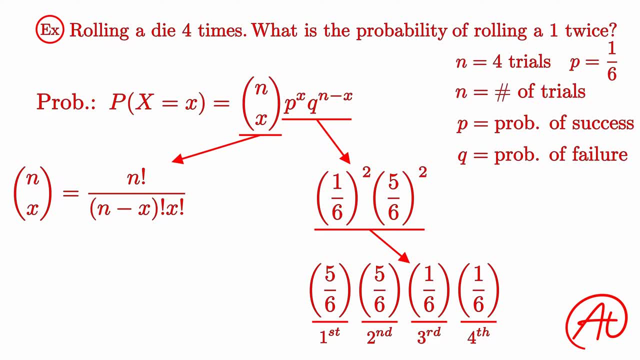 not as scary as it looks If you haven't seen them before. these exclamation points represent factorials, And all a factorial is is taking a number and multiplying it by each integer below it until you reach 1.. So the factorial of 3 would be 3 times 2 times 1, or equal to 6.. And if we wanted to calculate, 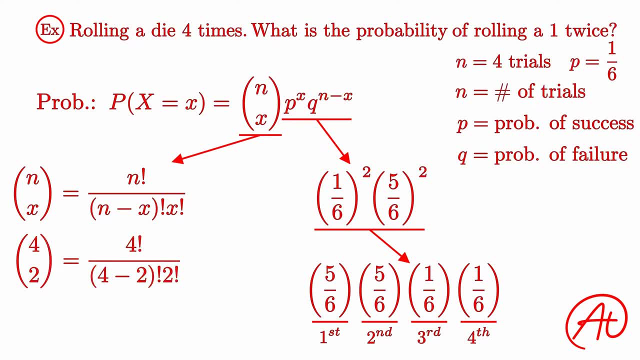 4, choose 2,. for our example, we would take 4 factorial and divide it by 4 minus 2 factorial times 2 factorial. As a result, our top would be 4 times 3 times 2 times 1, and our bottom? 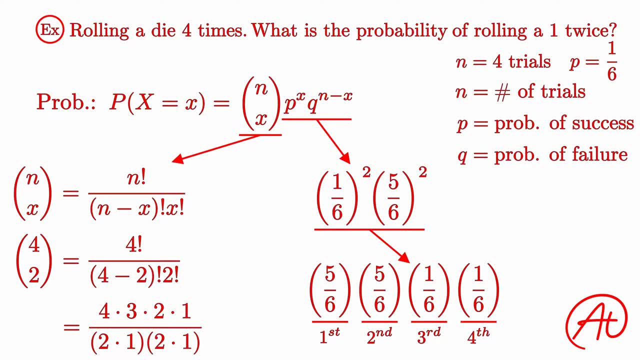 would be 2 times 1 times 2 times 1.. And this equals 24 over 4, or 6.. So this means that out of our 4 rolls, there are 6 different ways to roll a 1 twice Overall in order. 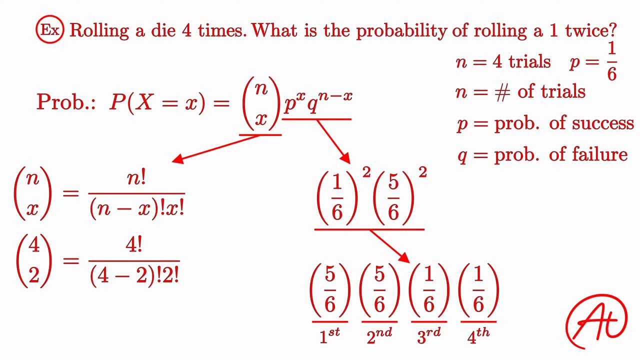 and divide it by 4 minus 2 factorial, And that's what we would get. We would get 2 factorial times 2 factorial. As a result, our top would be 4 times 3 times 2 times 1, and our bottom would be 2 times. 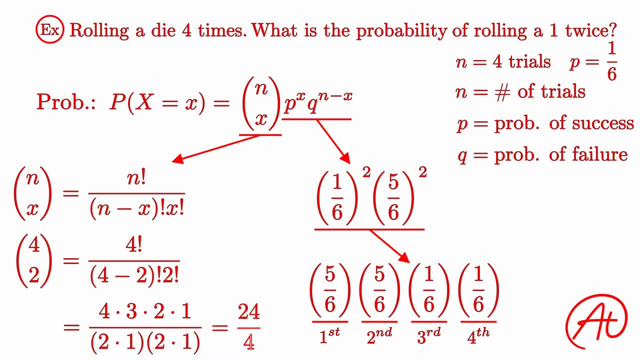 1 times 2 times 1.. And this equals 24 over 4, or 6.. So this means that out of our 4 rolls, there are 6 different ways to roll a 1 twice Overall. in order to find the probability of a 3 roll, you would need to add a minimum. 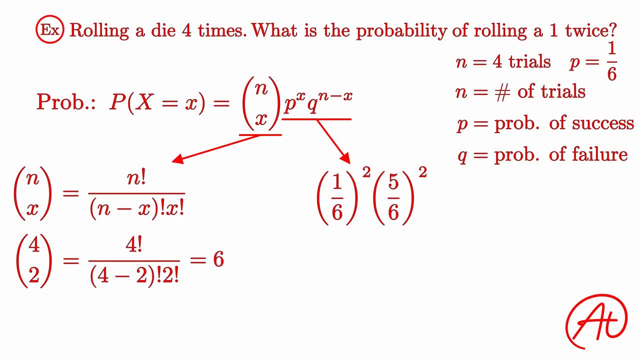 certain outcome. we take the probability of reaching that outcome in one specific way and multiply it by the total number of possible ways there are to write that desired outcome And to see it in its full beauty. the probability of rolling two ones is equal to 4. choose 2. 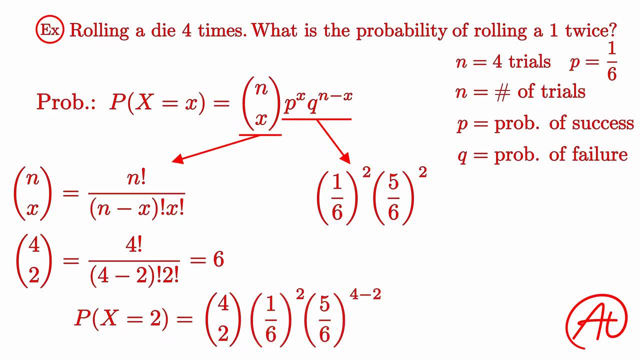 times 1 sixth squared, times 5 sixths, raised to 4 minus 2.. Using our previous calculations, this simplifies to: 6 times 1 sixth squared, times 5 sixths squared, or 0.1157.. So the probability of rolling one twice in four rolls is 11.57%. 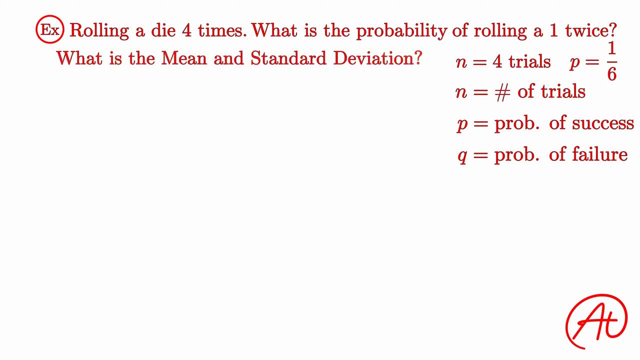 And just for fun, let's also find the mean and standard deviation of this scenario. Once again, to find the mean, we multiply n times p, Or for our example, 4 times 1, sixth, to get that mu equals 4 sixths. 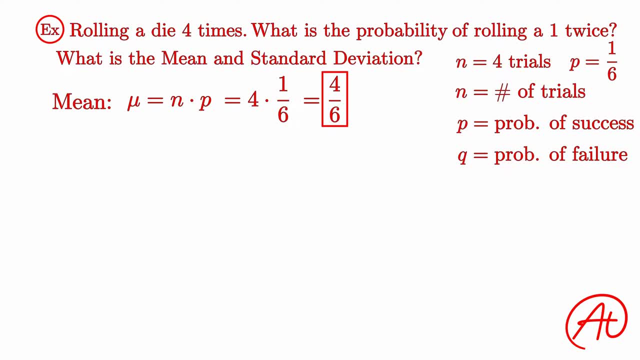 And what this means is that during your four rolls you can expect to roll a one, 4 sixths times- And this might seem a little strange because you can't roll a one, 4 sixths of a time. But if you were to repeat this experiment of four rolls again and again and average, 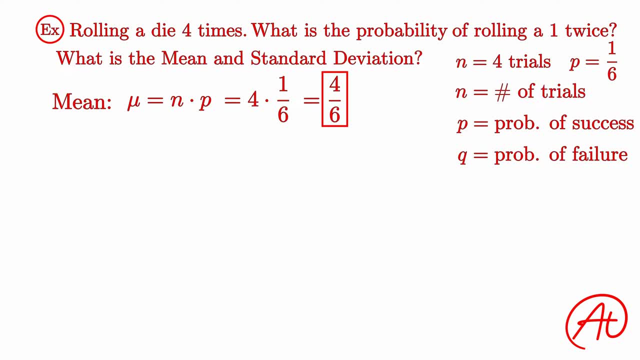 the number of times you've rolled a. one per experiment. the value you get would approach 4 sixths. Next, to calculate the standard deviation, we would take the square root of n times p, times 1 minus p, Which would be the square root of 4 times 1 sixths. times 1 minus 1 sixths. 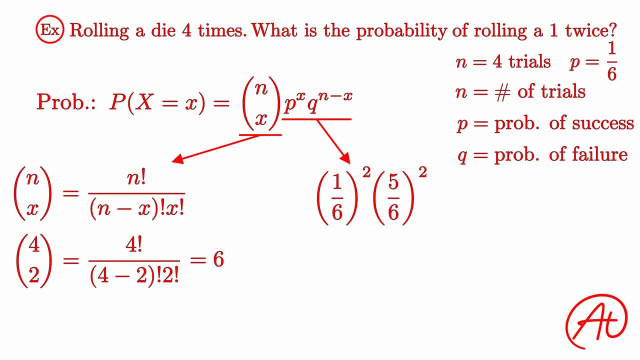 to find the probability of a certain result. we need to find the probability of a certain outcome. we take the probability of reaching that outcome in one specific way and multiply it by the total number of possible ways there are to write that desired outcome And to 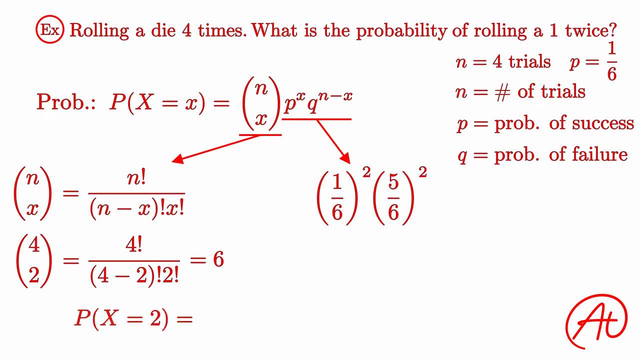 see it in its full beauty. the probability of rolling two 1s is equal to 4. choose 2 times 1. sixth squared times 5, sixths, raised to 4 minus 2.. Using our previous calculations, this simplifies to 6 times 1. sixth squared times 2 fifths: This simplifies to 4. choose. 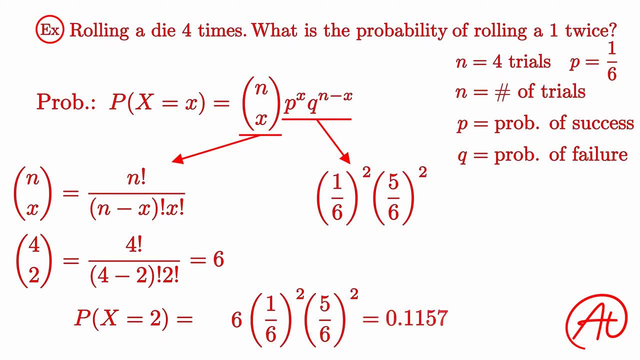 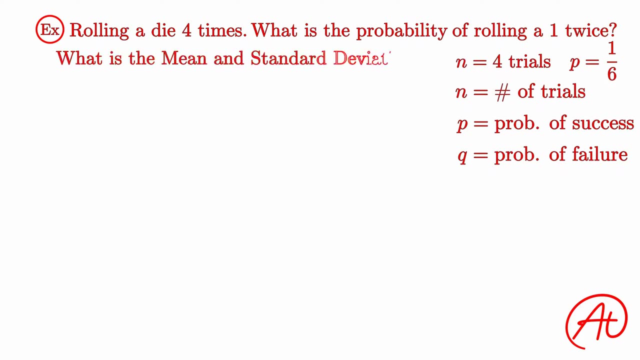 squared times 5, sixths squared, or 0.1157.. So the probability of rolling 1 twice in 4 rolls is 11.57%. And just for fun, let's also find the mean and standard deviation of this scenario. 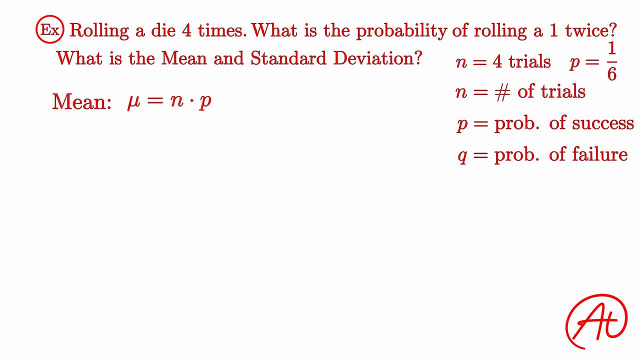 Once again to find the mean. we multiply n times p, or, for our example, 4 times 1 sixths, to get that mu equals 4 sixths, And what this means is that during your 4 rolls you can expect to roll a 1, 4 sixths. 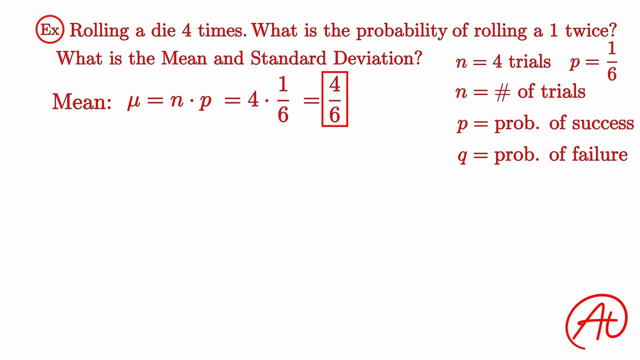 times- And this might seem a little strange because you can't roll a 1 4 sixths of a time. but if you were to repeat this experiment of 4 rolls again and again and average the number of times you rolled a 1 per experiment, the value you get would approach 4 sixths. 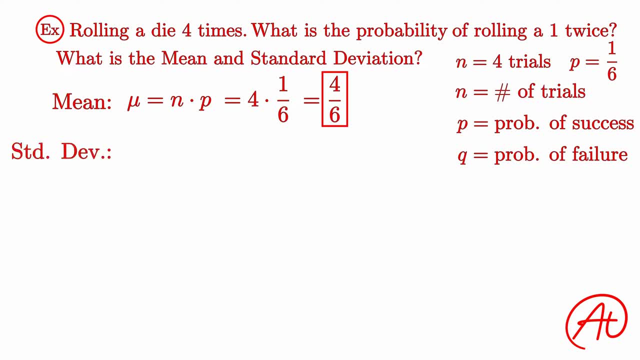 Next, To calculate the standard deviation, we would take the square root of n times p times 1 minus p, which would be the square root of 4 times 1 sixths times 1 minus 1 sixths, or 4 times 1 sixths times 5 sixths, or equal to 0.745.. 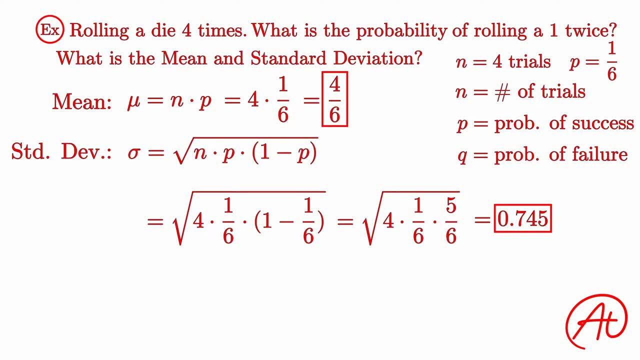 Now I hope you found this video helpful in your journey to master statistics, But if you have any questions or feedback for how we can make our videos better, please let us know down in the comments. And if you did find this helpful, please tap those like and subscribe buttons to see more. 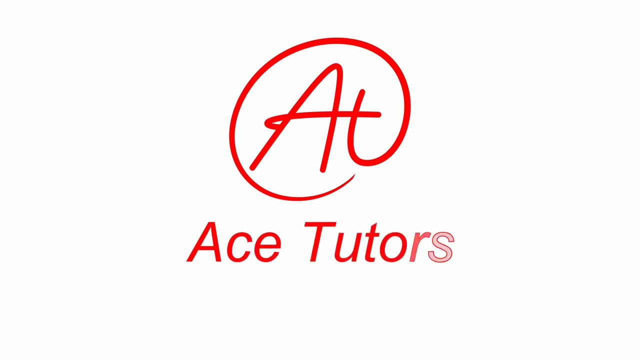 of our content. Thanks again for watching and remember you have big dreams. don't let a class get in the way.